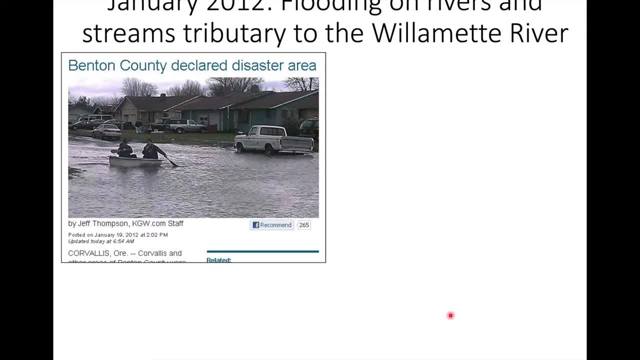 from where I lived. From what I can tell, my house would have been dry basement around here, but I would not have been able to leave the house during this flood. The stream that my neighborhood was near didn't have a stream gauge on it, so I went looking. 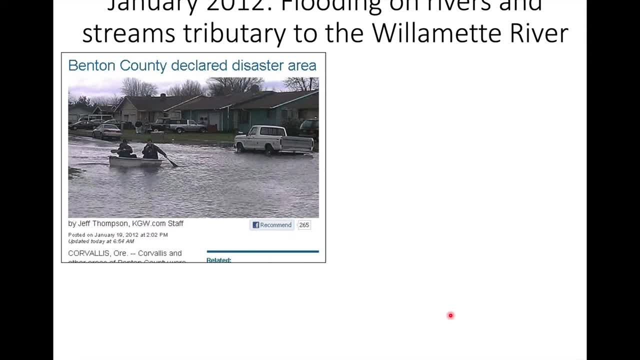 for the closest river that did have a USGS stream gauge, and that is the Marys River, which comes into the Willamette in Corvallis, And a friend who still lived in the area in 2012 took this picture of flooding along the Marys River. 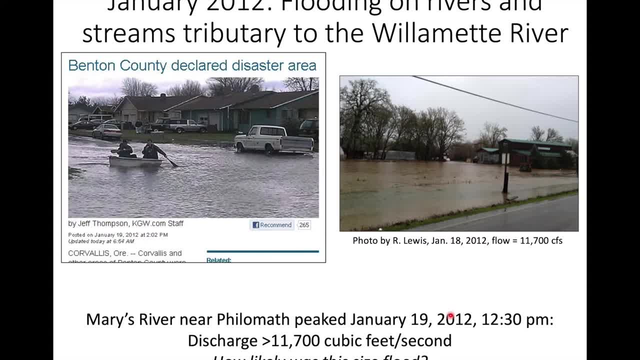 Near the peak stream flow. So the Marys River near Philomath, just outside Corvallis, peaked at about 11,700 cubic feet per second And the question I had when this event was happening is: how likely was this size of flood on the Marys River? It was certainly unprecedented in my 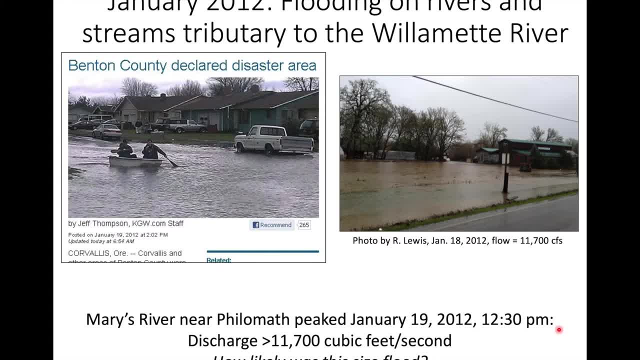 neighborhood and again, I know that was the hardest-hit area, but more widely in the region, was this an extraordinary event Or was this kind of run-of-the-mill? So we're going to go back in time now to late January 2012,, when I was downloading. 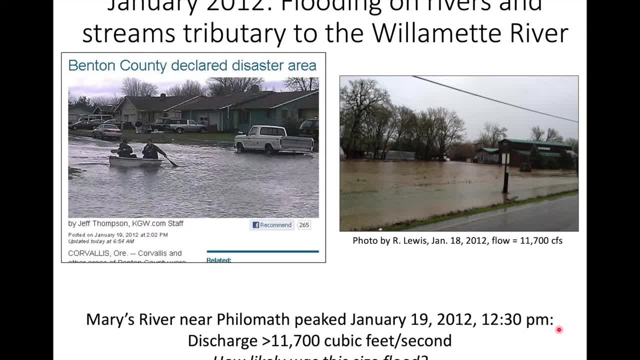 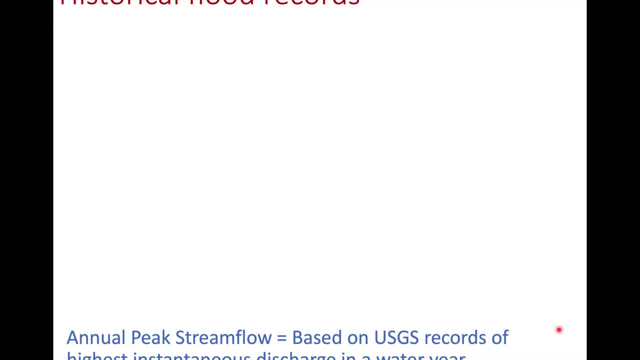 the data from the USGS and trying to figure out the answer to this question. So to start a flood frequency analysis, you use historical flood records And the type of data you look at is called the annual peak stream flow time series. And so when you go to the USGS website, 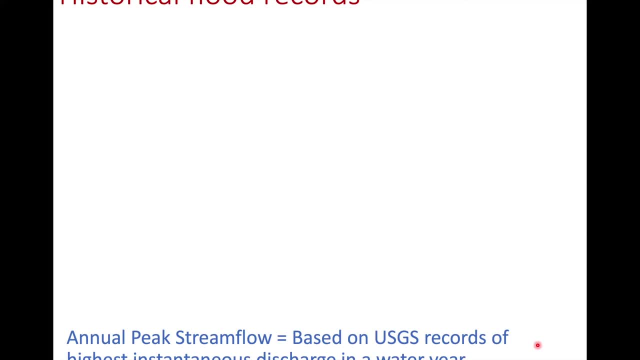 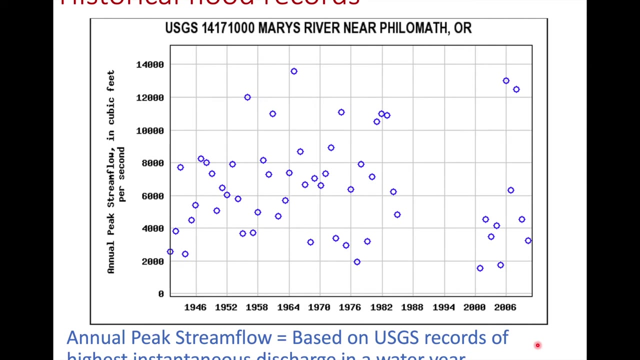 this time series gives you the highest instantaneous discharge measured in a water year, So the single measurement in a whole water year where flow was highest at the gauge, So annual peak stream flow. And when you download it from the website it looks like this: 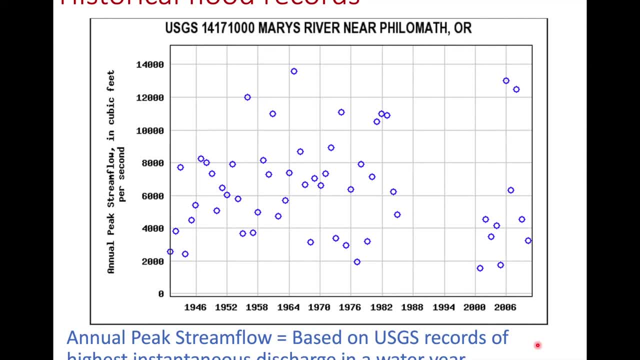 So this is the Marys River near Philomath as of 2012.. And we can see that the gauge operated since the 1940s. There's kind of a gap in the 1990s and then it picks up again in about year 2000.. 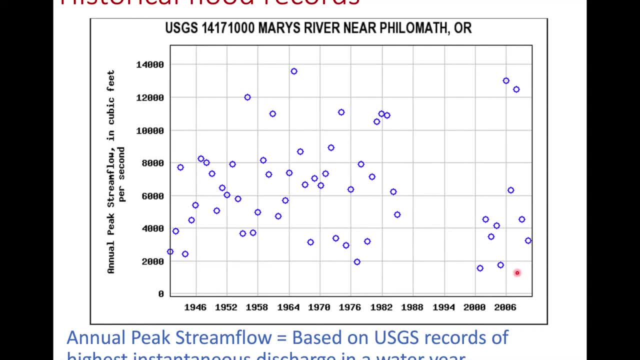 So the peak stream flow was 11,700 cubic feet per second And just by eyeballing it we can see that's not an unprecedented event. It's certainly been encountered in the past. But if we want to formalize this and find out what the probability of this size flood happening in any given year is, 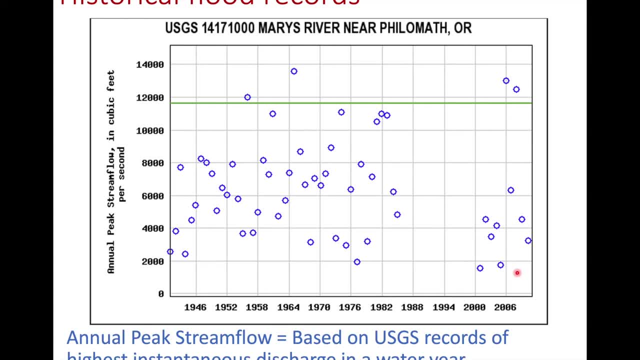 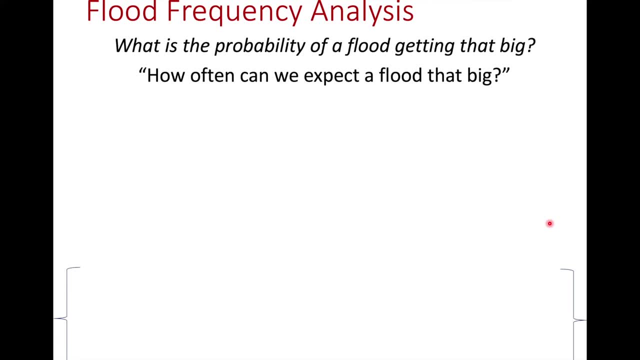 then we need to go the next step into the flood frequency analysis. So flood frequency analysis answers the question: what is the probability of a flood getting to be that big? Oftentimes we frame this in terms of how often can we expect a flood to be that big? 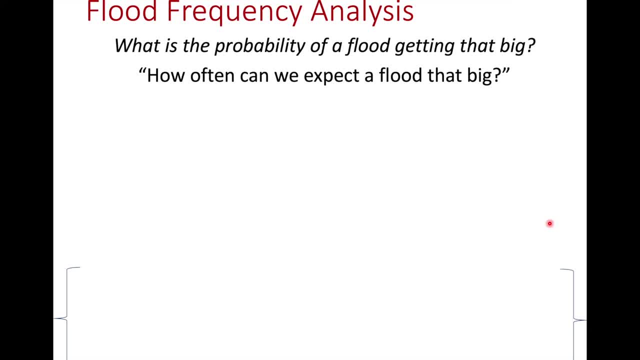 And we'll talk in a few minutes about the difference between a probability and a recurrence interval and why thinking about these things in terms of a likelihood or a probability is better than thinking about them in terms of a recurrence interval. OK, so how do we do this? 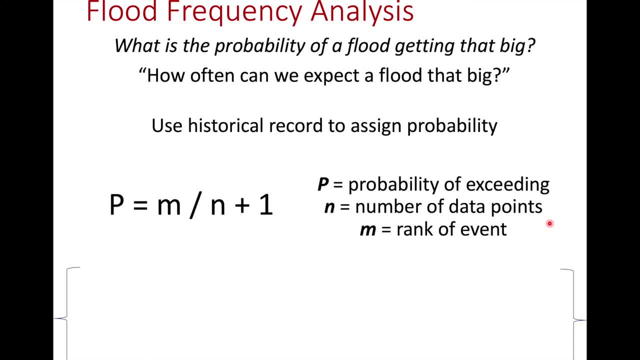 We take that annual peak stream flow record and we assign probabilities to them. If you've created a flow duration curve, this formula will look familiar. We take all of the points in our historical record. We rank them from biggest to littlest, We assign them a rank and then we divide by the number of points in the record plus one, and do that math. 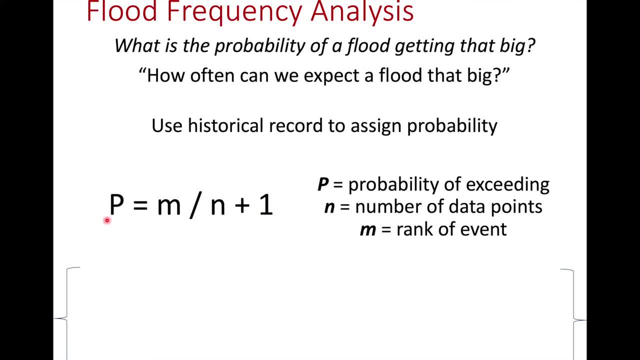 And we get a probability for each event Before we start to plot- We're going to start to plot blindly through some numbers from the USGS into a flood frequency analysis- that we need to stop and ask ourselves some questions like: are the events independent and random? 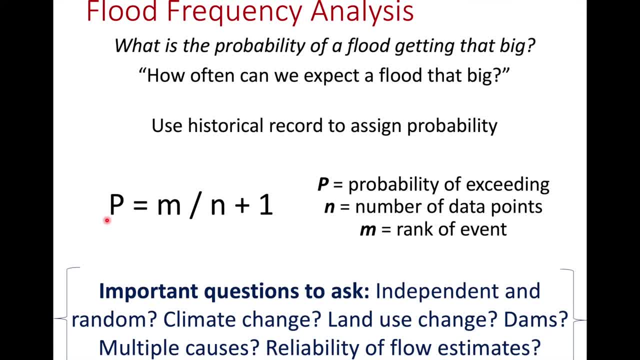 That is actually why we take only the largest stream flow of each water year, because we wouldn't want the same flood to be counted twice. The second thing is: is there climate change or land use change occurring in the watershed that could make our data? 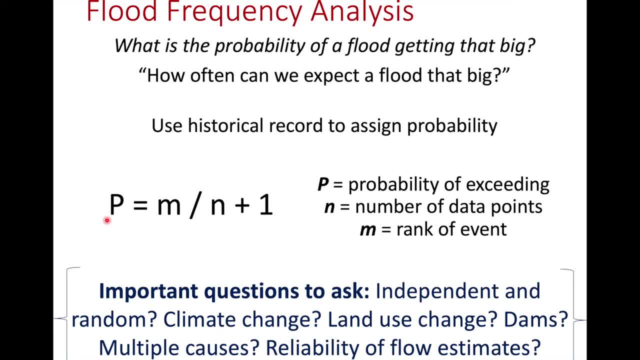 Our data not really represent the conditions we're interested in going forward, For example, the dams going in on the Willamette River. Are there multiple causes of floods And we might need to think about some floods as not belonging to the same statistical distribution as others. 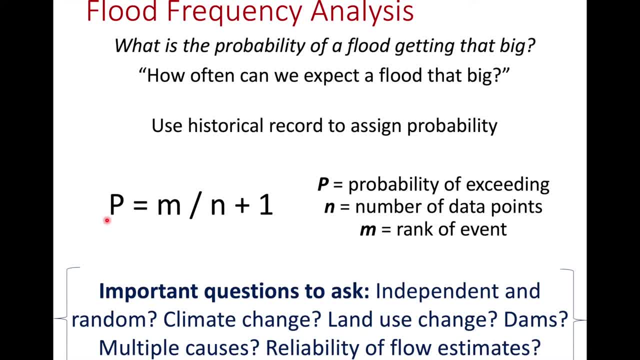 For example, if you had a dam break flood, we might think: hope that that's a one off event And we shouldn't include that flood in an analysis. OK, So we're going to look at that flood in an analysis. that's really much more interested in the probability of different sizes of floods associated with rainfall. 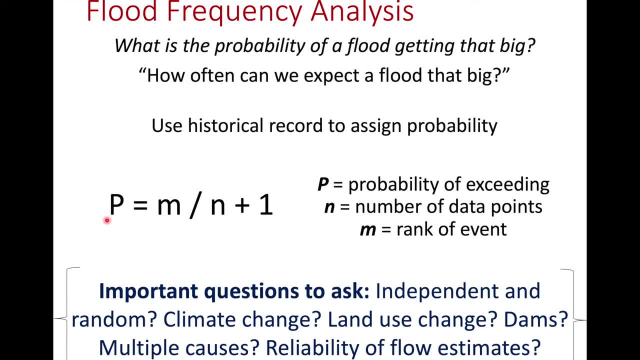 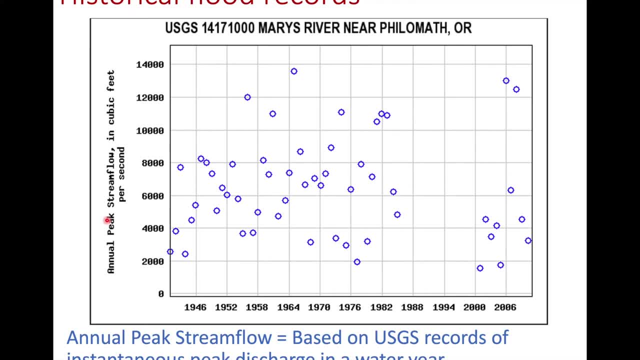 And then finally, how reliable are our flow measurements at these really high flows? All right, So we're going to ask ourselves all these questions when we download the data. We're going to especially look at things. if there are gaps, Use what we know about the watershed and the history of the watershed. 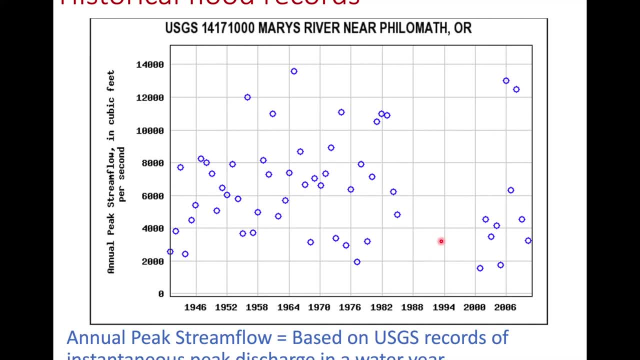 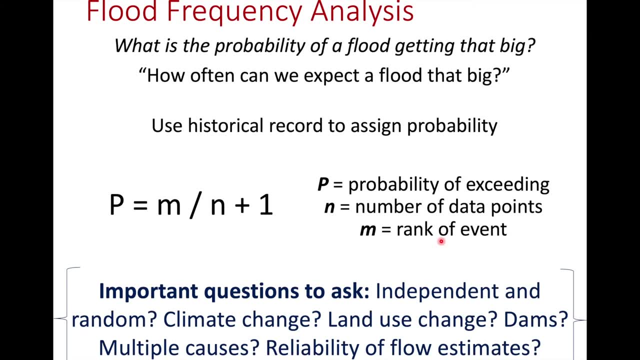 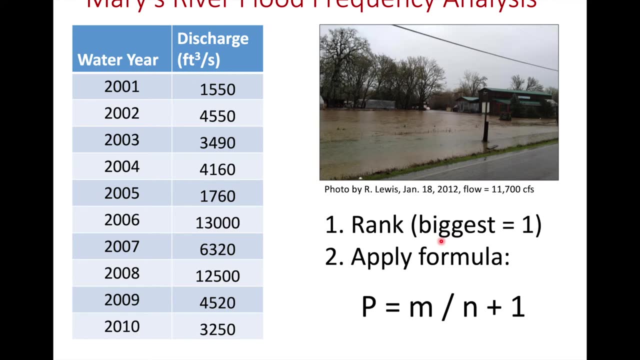 And then we're going to decide how much of the streamflow record we can actually use in our flow frequency analysis. For this one we could probably use the whole record, But we could also simplify it down to just the period that was published, in the 10 years between when the gauge restarted and when the flood that we're interested in occurred. 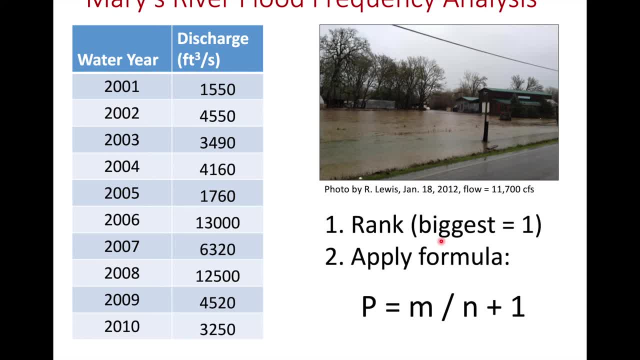 And that will make things fit a little bit easier on the PowerPoint screen. So here's a walkthrough example of a flood frequency analysis for the Marys River. So if we look at the data, we have one flood per water year. Here's our discharge. 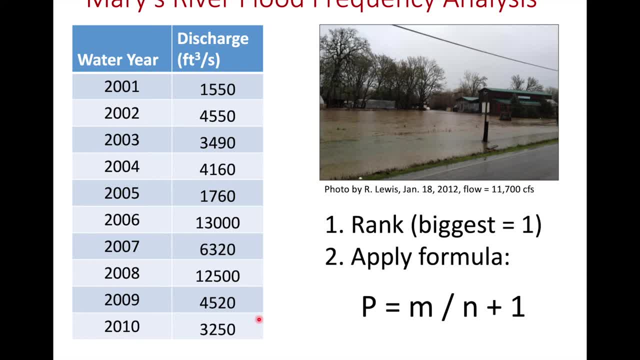 We're going to stick with cubic feet per second for the purposes of this PowerPoint. We're going to rank them from biggest to littlest, And then we're going to apply this formula to calculate probability. All right, So I've done that. now. 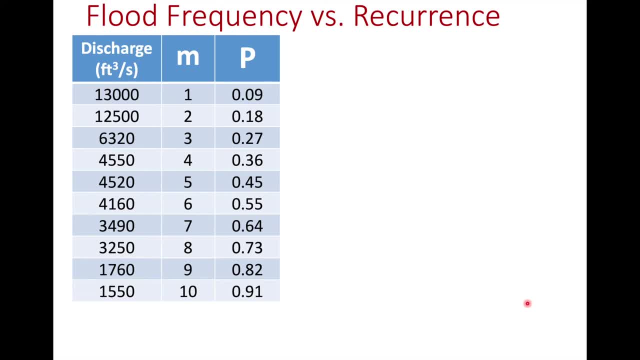 I've gotten rid of the water year because when it occurred is not what we're interested in. We simplified it, So we simply want to know how big it was, That's this column, And what the probability of them is. All right, 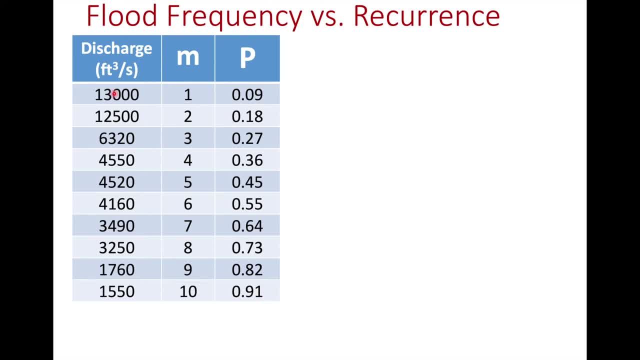 So those two columns, probability and discharge, are the main ones we're going to use in the flood frequency analysis. But before we get there, let's talk a little bit about this idea of recurrence interval, And this is what we talk about when we say something like the 100-year flood, or the 500-year flood, or the two-year flood. 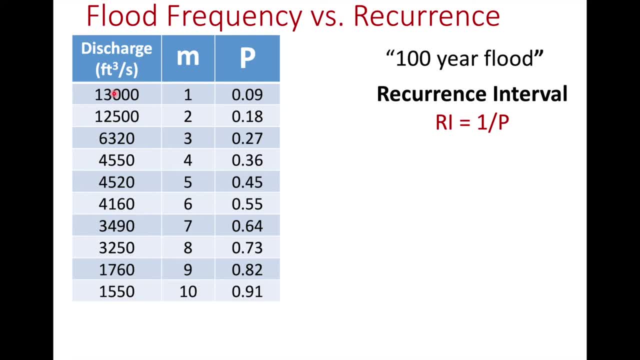 And all that is really doing is taking one over the probability. All right, So the recurrence interval is one over the probability. So if we have a probability of 0.09, our recurrence interval is 11 years. Notice that the longest recurrence interval we can get is just one year longer than the streamflow record that we're analyzing. 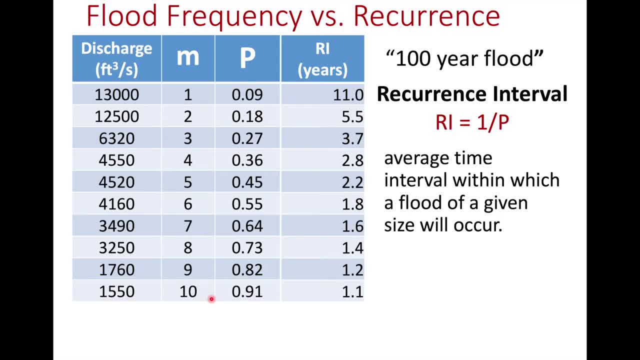 All right, But the probability and the recurrence interval being linked means that this is going to be one year longer than the streamflow record that we're analyzing. All right, But the probability and the recurrence interval being linked means that this is really just telling us the average, the sort of most likely time interval within which a flood of a given size will occur. 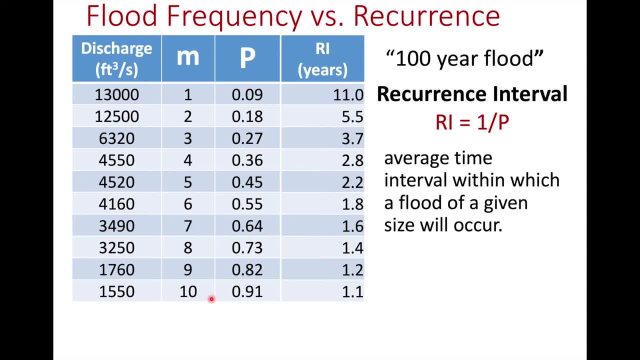 All right, It doesn't tell us that 11 years after the last 13,000 cubic foot per second flood, we can expect another one. It's not a return period. If you had a 100-year flood on your river last year, unfortunately you could have a 100-year flood. 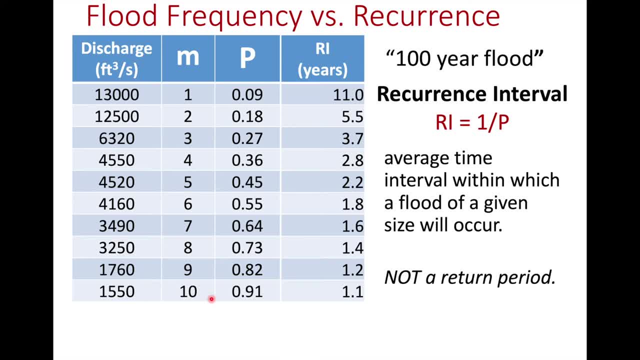 All right. So if you could have a 100-year flood on your river next year, it just says that in any given year these are independent events, that a 100-year flood has a one over 100 probability, a 1% probability. 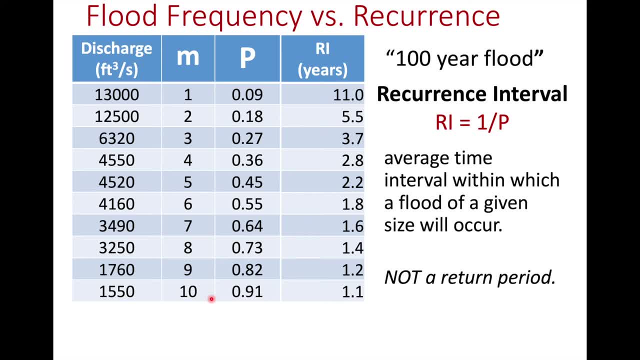 All right, And so you should be really comfortable thinking about these floods in terms of probabilities and communicating them in terms of probabilities, even though you will hear other people- the news media, politicians- say that they're not 100-year floods. All right. 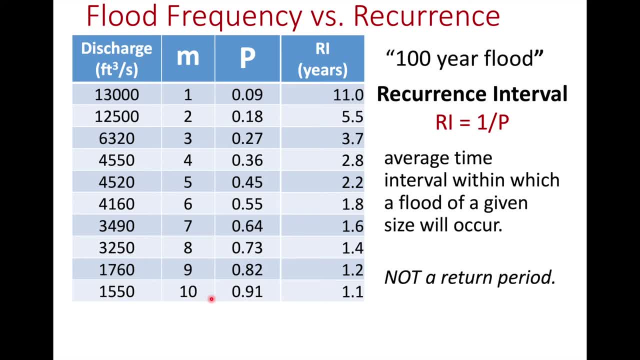 So this is really just telling us that this is a 100-year flood. This is a 100-year flood. This is a 1 over 100 probability, All right. So the reason we think of these floods is because they're independent events. 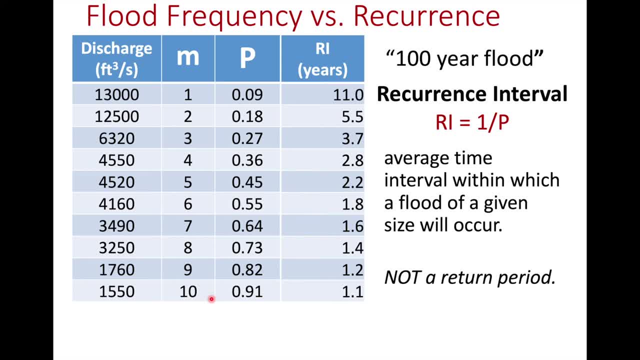 politicians, the general public, talking about things as recurrence intervals. But in order to avoid misconceptions that just because someone's house didn't flood in the 1964 flood- and that was a hundred year flood, therefore they're safe till 2064,, it makes sense to talk about these. 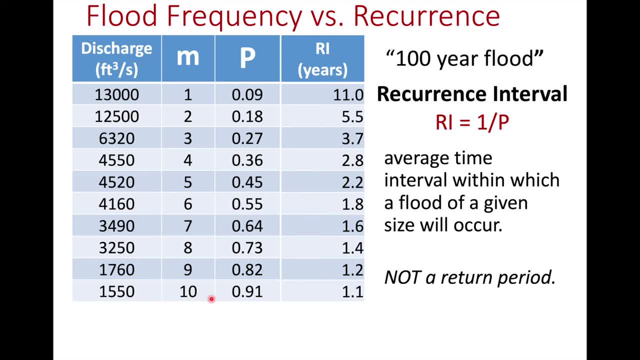 things in terms of probabilities as often as we can. If you want this written out a little bit more for you, I have a blog post about why you can get a 500 year flood two years in a row. All right, for now, though, let's focus on the science and the math. 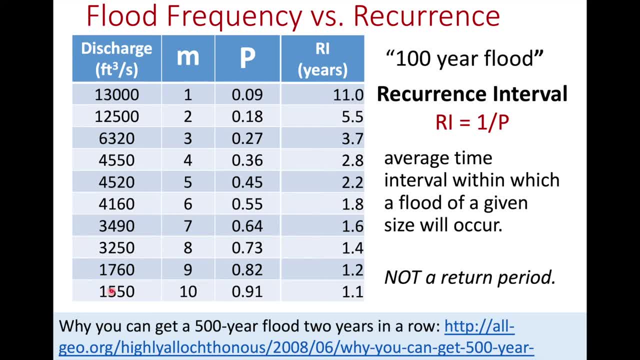 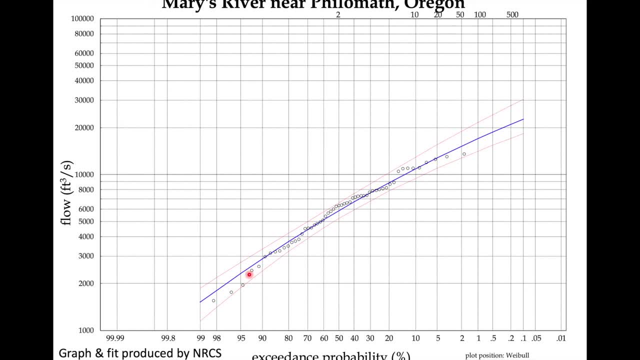 So we're going to now plot up our discharge versus our probability And we can get a graph like this. So each one of these plots- and now I didn't just use 10 years, I used the whole record for the Marys River because, again, I feel pretty comfortable that- 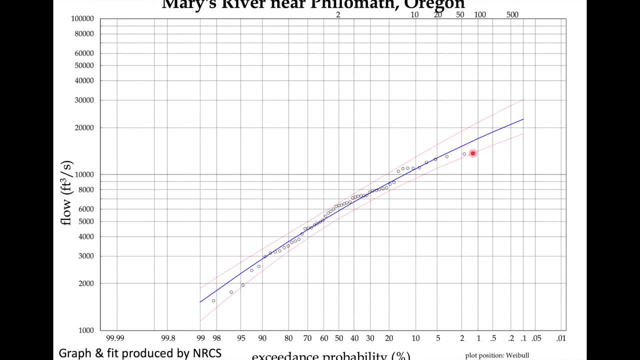 there have been no dams built on the river. The watershed land use has remained more or less the same. It appears to all be part of the same statistical distribution, So I'm going to include it all in my analysis. So all of these plot points are fitted up. They represent one. 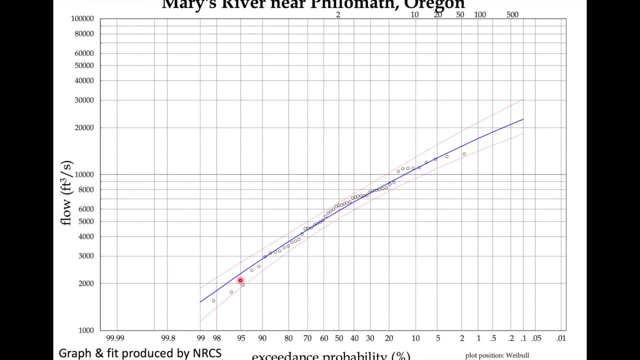 of the largest events per year. All right, And then we are going to fit a line through our points. Now, if you're in my class, you're going to do this by hand, By eye, but we can also choose a statistical distribution to fit the line, And one that is: 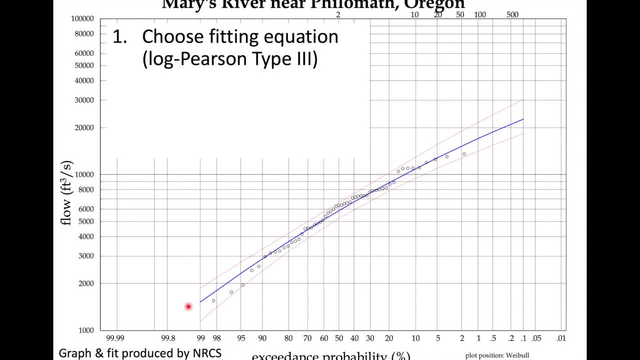 really commonly used in the US and used by the US Geological Survey, is called the log Pearson type three, And if you go on in hydrology it's worth learning that method. The other thing, another thing to notice about this graph is that we can put uncertainty bounds. These are these red lines. 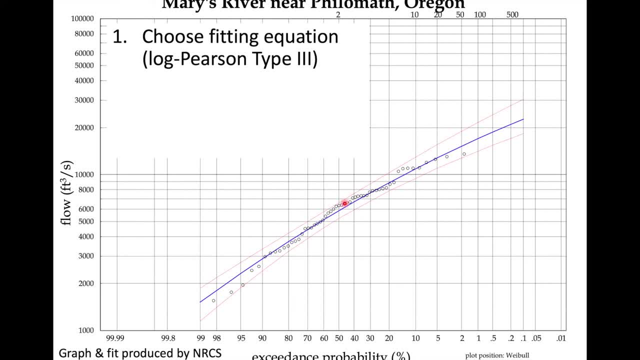 on either side of our data And notice that we have less uncertainty where we have a lot of data and we have more uncertainty where we have less data. And so we can again, if we're being really good and careful communicators, rather than saying that, say, the 10 year recurrence interval, flood or the 10%. 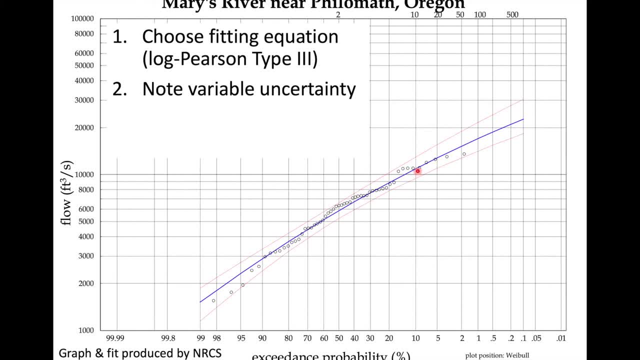 exceedance probability: flood is exactly 10,500 cubic feet per second. We would instead talk about it as over a range. So if we take that example, we would instead say that it goes from about 9,000 to 11,000 cubic feet per second as a good range of a 10% probability. 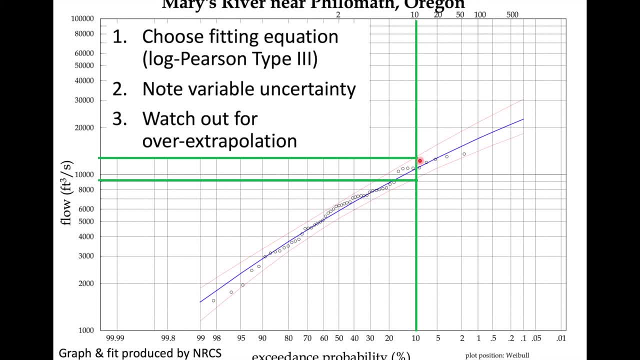 flood for the Marys River. All right. Another thing when you're looking at data like this is to watch out for over extrapolation. If somebody came to me and said I can tell you what the 500 year flood looks like on the Marys River because I've plotted it up and fit a, 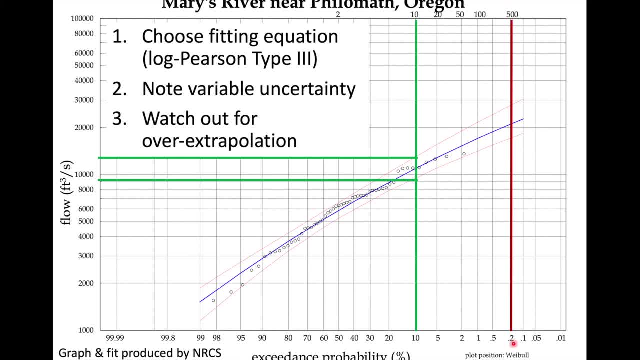 distribution, I would say well, the 500 year flood, the 0.2% probability flood, is way out beyond the range of our data. How confident do we really feel that a flood that occurs that infrequently we understand and can put good estimates on? So we can extend way beyond the. 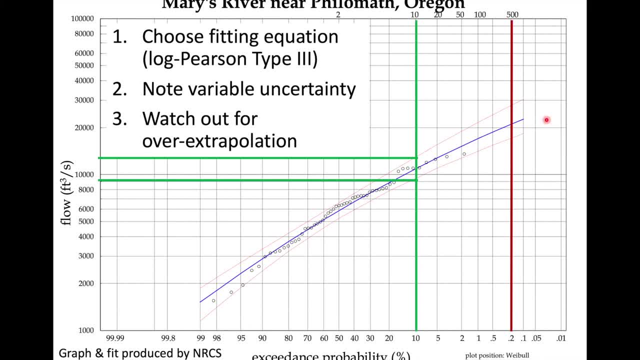 range of the data. But anytime you hear a politician or a politician say, oh, we don't know where the media are talking about 500 year, 1,000 year events, you should take that with a pretty big grain of salt. because of these large uncertainty bands And because in North America 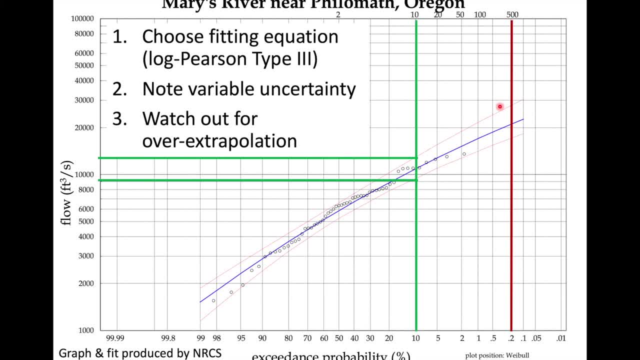 we have very few records that extend even beyond 100 years, And many, many records are much, much shorter. All right, So that is what a basic flood frequency graph looks like, What sorts of information you can use to measure flood frequency. 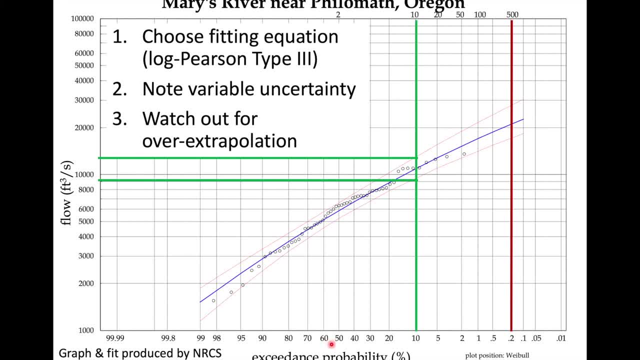 And you can get from it. So you can then use the line fitted through your data to give an estimate of a flood of any particular probability that you're interested in. So if you're interested in the 50% exceedance probability, you would go up to that line. read over across the graph. 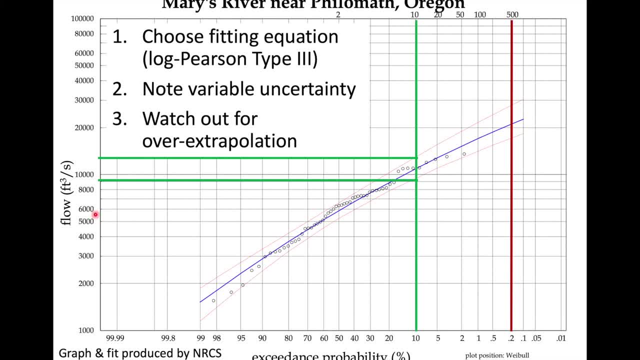 and you would say it is just below 6,000 cubic feet per second. Or if we're being good, we would say it's between 5,000 and about 6,500 cubic Feet per second. And we could do that for the 1% flood or 100 year flood. read over the same thing. 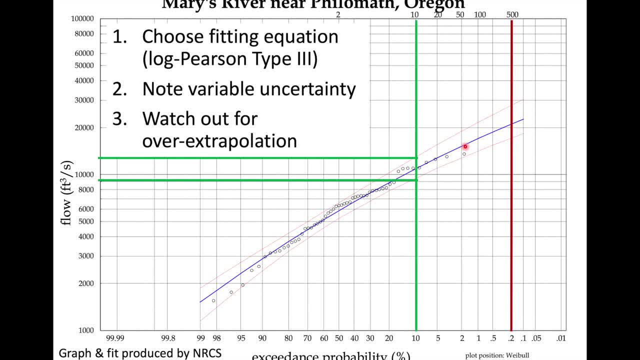 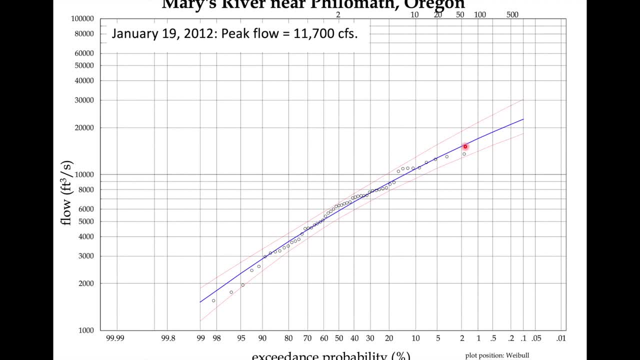 But where does our January 2012 event fit in? Okay, Back to the data. It was 11,700 cubic feet per second, And so we can go over from there and then down And we see it's about a 6% exceedance. 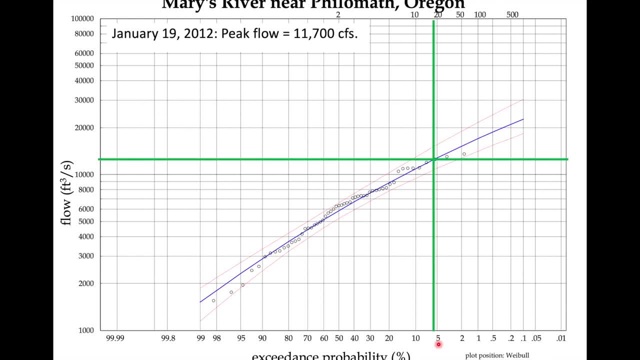 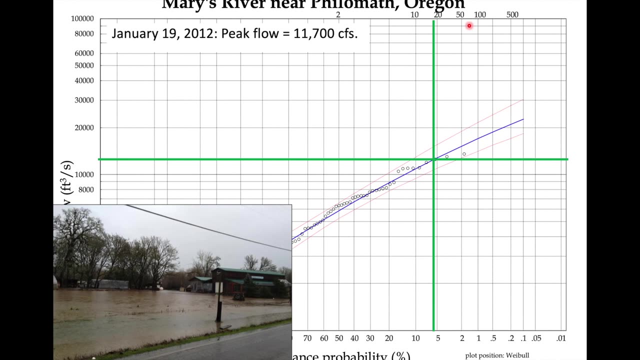 probability, And if we wanted to put that into a recurrence interval, it's a little bit less than a 20 year recurrence interval on the Mary's River near Philomath. And so now if we go back to our flooded farm there, this is actually probably a pretty good land use, So there are some farm buildings.